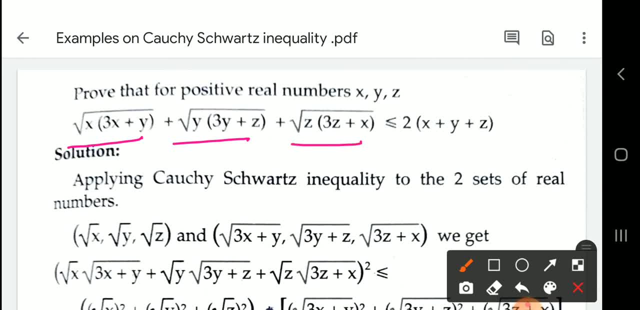 example. So let us see the example. So let us see the example. So we apply here Cauchy-Scott's inequality for the two sets. Here we see the two sets, which are root x, root y, root z and root of. 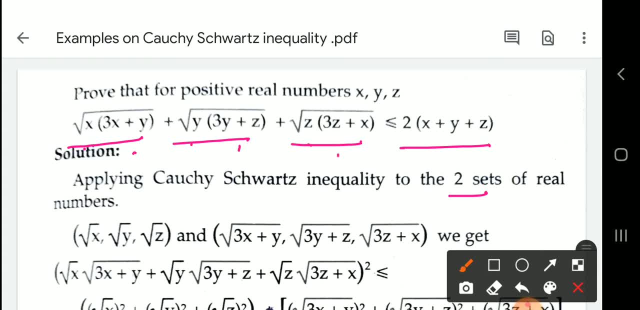 3x plus y, root of 3y plus z and root of 3z plus x. So we applying Cauchy-Scott's inequality for these two sets. Okay, So this is our a 1, b, 1.. Okay, a 1, a, 2, a, 3. and here b 1, b, 2, b, 3.. Okay, we apply this. 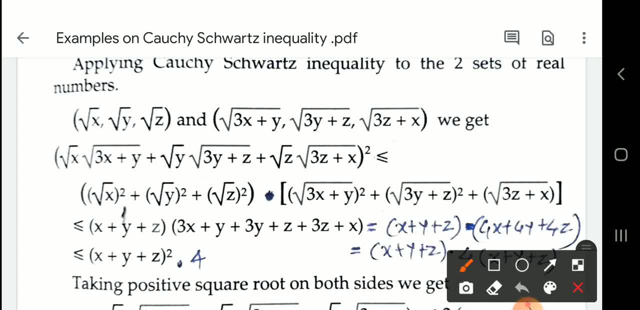 Cauchy-Scott's inequality. So applying that inequality we get here. Okay, left hand side guy, summation i running from 1 to n: a, 1, b, 1 plus a, 2, b, 2 and so on. or summation i running: 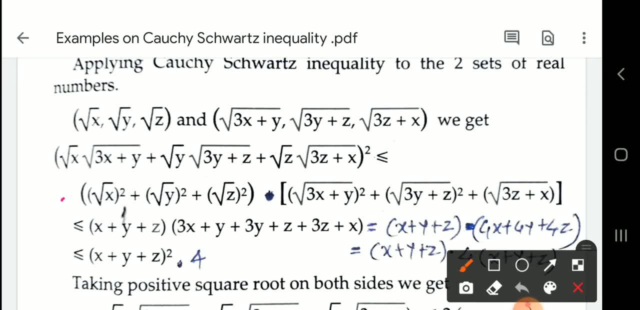 from 1 to n, a, i, b, i bracket square. Okay means two sets: a 1, b 1 plus a 2, b 2 plus a 3, b 3, and so on. Okay. so this is our a 1, b 1. okay, a 1, b 1 plus a 2, b 2 plus a 3, b 3, and so on. 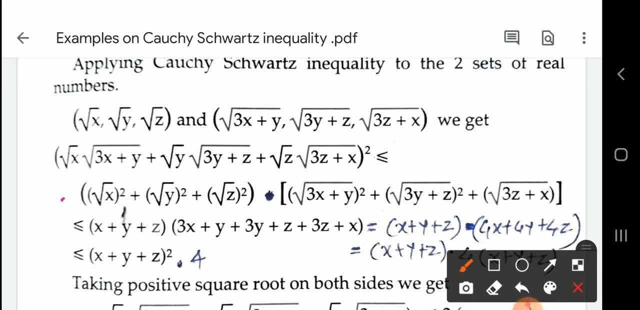 Okay, that means lhc is a 1, b. 1 means root x into this term plus root y into this term plus root z into this term. Okay, the square of all this. Okay, this term is less than or equal to Cauchy summation. i, running from 1 to n, a i square, I mean we make all a i. 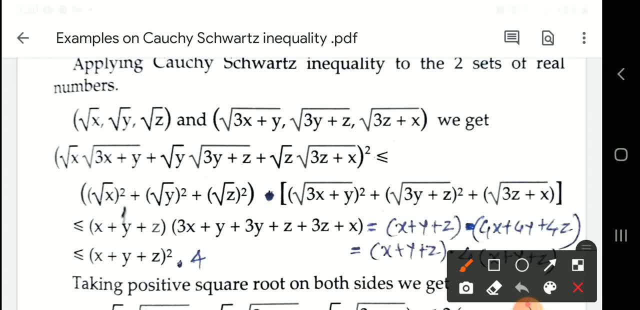 square and then we sum them Meaning what we will get is root x- bracket square plus root root y bracket square plus root z bracket square. okay, into summation i: running from 1 to n by square means all b, all these terms square: b1 square plus b2 square plus b3 square. that means 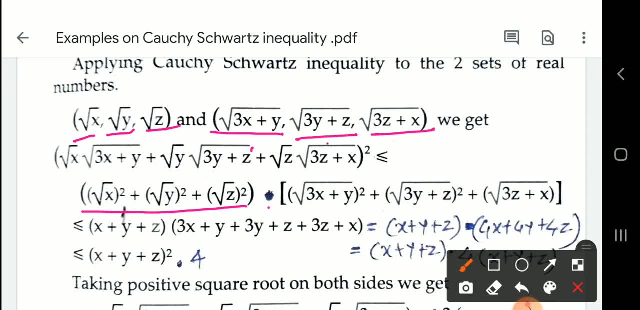 root of 3x plus y square plus root of 3y plus z square plus root of 3z plus x square. the square term right here, 3z plus x square. okay, so here we get. our alias is so this term is less than or. 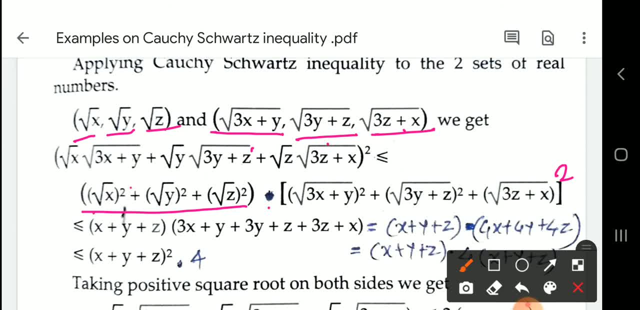 equal to. we solve this term okay. i just now root x, square x, root y. square is y. root z. square is z. that means this bracket: after simplification, we get x plus y plus z and here again square and square root. cancel one. that means 3x plus y plus 3y plus z plus 3z plus x. 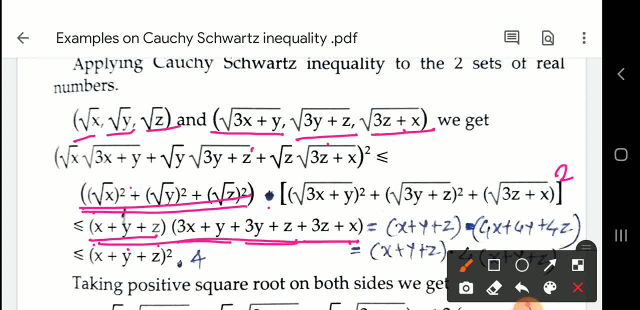 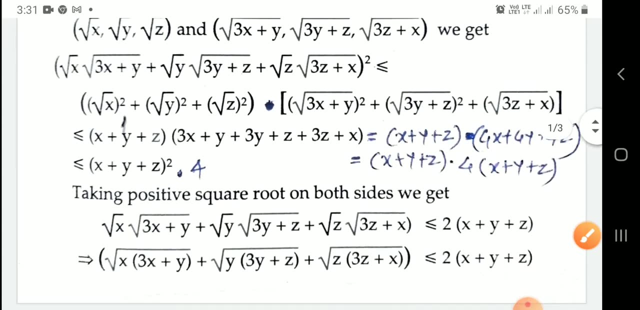 okay, okay, by solving this term, we get here 3x plus x, that means 4x, y plus 3 by 4y, and z plus 3z is 3z, that means we get here x plus y plus z into 4x plus 4y plus 4z, taking four common from: 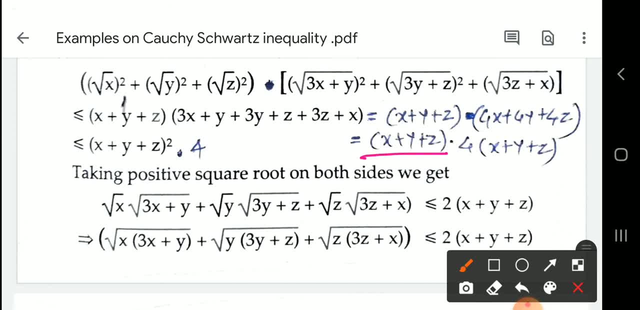 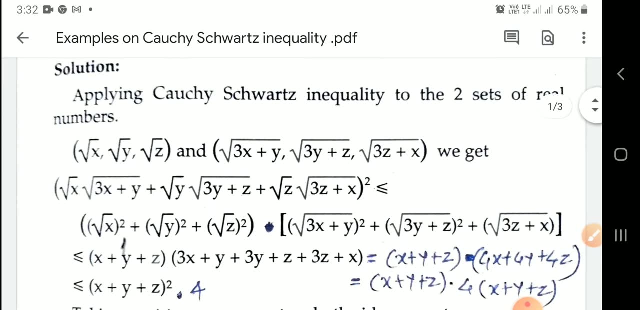 each term. here we get x into y into z, into 4x plus y plus z. that means we get 4 into x plus y plus z, bracket square. ok, that means we get here root x into root, x into root of 3x plus y plus root. y. 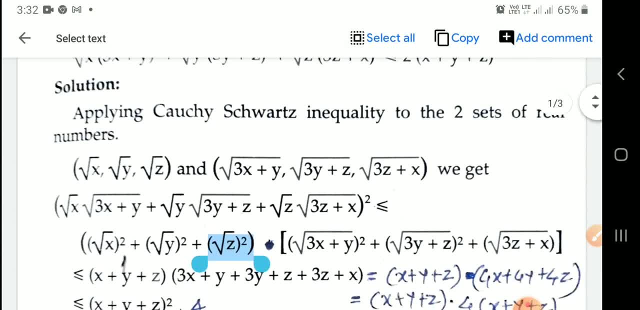 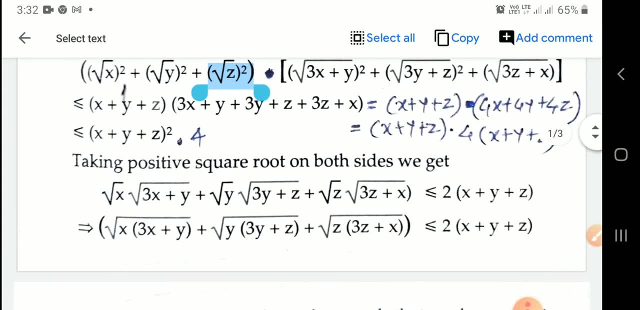 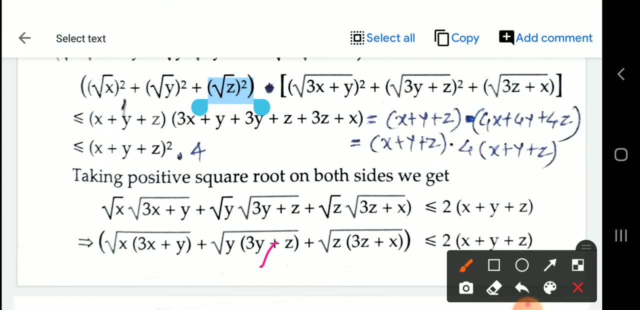 into root of 3y plus z plus root z into 3z plus x square. this term is less than or equal to this term is less than or equal to here. we get here: root 4 jest ok. 4 into x plus y plus z bracket square. so now taking square root. 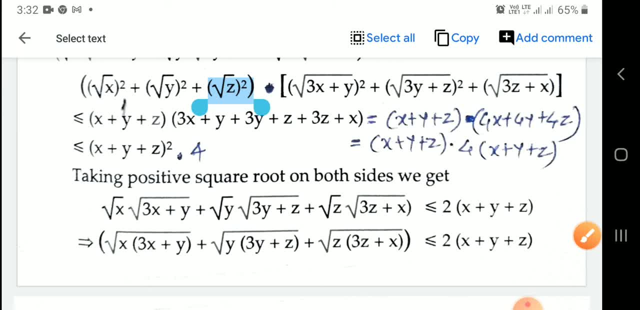 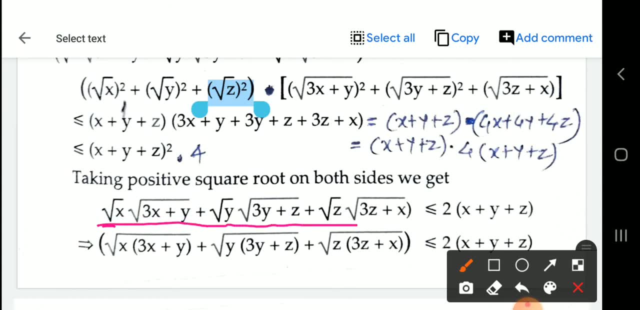 on both sides. we will give square root of both sides and here square cancel. Naval ok, so square cancel. after this we get taking square root from both sides. here is square cancel, here square root of this term: x plus y plus z, square root. we cancel it and square. 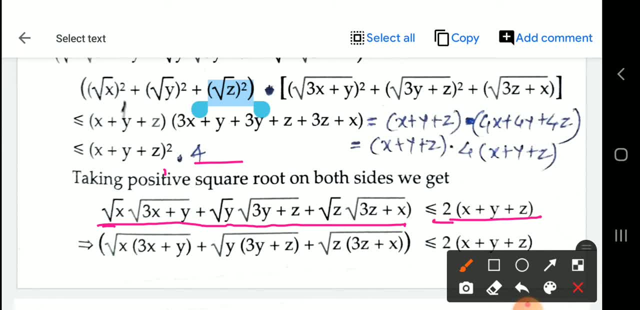 root of 4 is 2. ok, Kemal Raman, you will get 2 x plus y plus z square root, and square root of 4 is 2. ok, Now multiplication of root A into root B. You all of you know that. 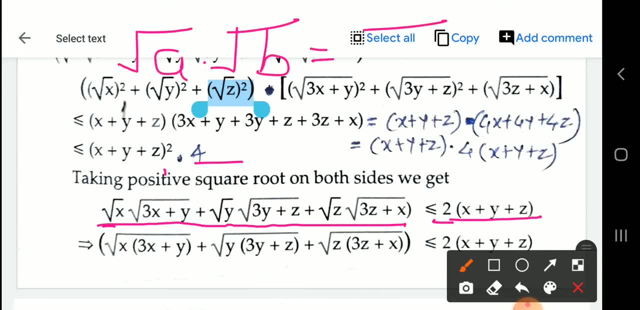 Root A into root B is equal to what Root of AB. So I mean root X into root of 3X plus Y, is root of X into bracket 3X plus Y, Y, root of Y into bracket 3Y plus Z plus root of Z into bracket 3Z plus X. 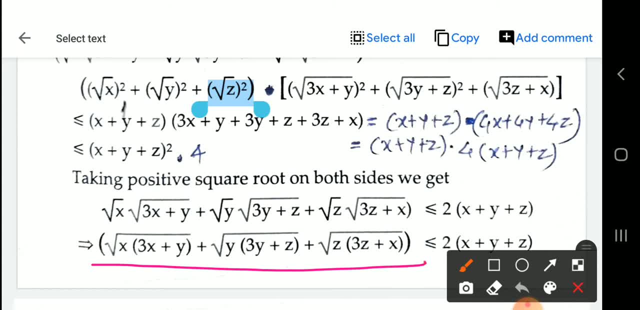 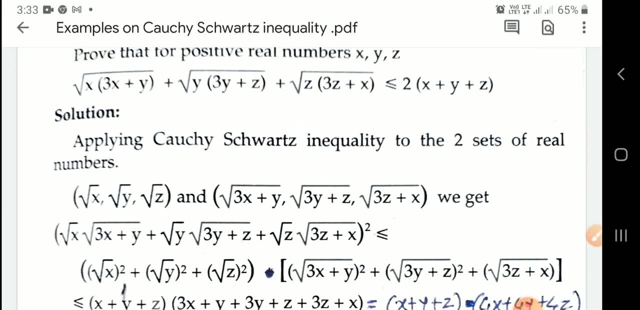 This term is less than or equal to this. So it is very, quite simple example: We are applying only Cauchy-Squad's inequality to these two sets. It is X, Y, Z and 3X plus Y, 3Y plus Z and 3Z plus X. 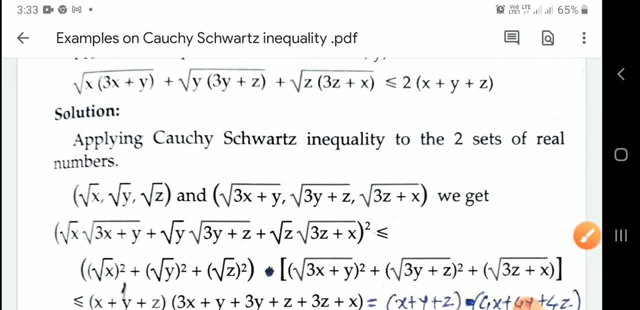 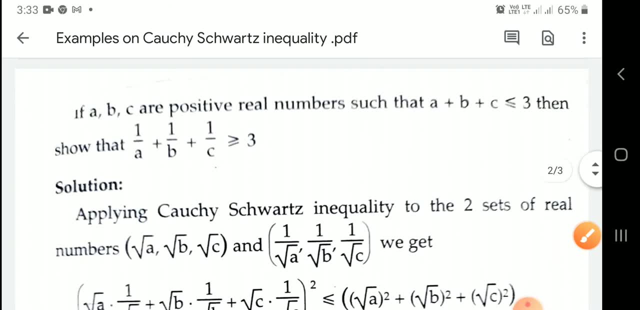 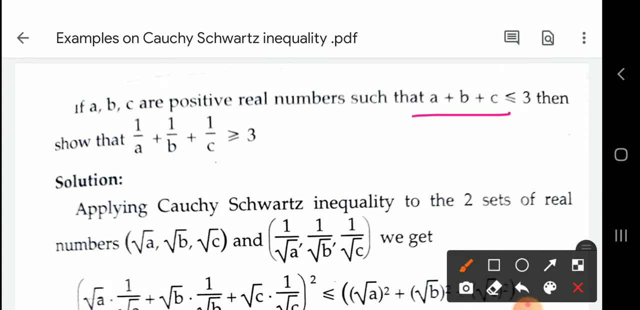 Okay, So it is very simple example. Solve it again. Okay, Now consider one more example. If A, B, C are positive real numbers, A, B, C are positive real numbers, Such that A plus B plus C is less than or equal to 3.. 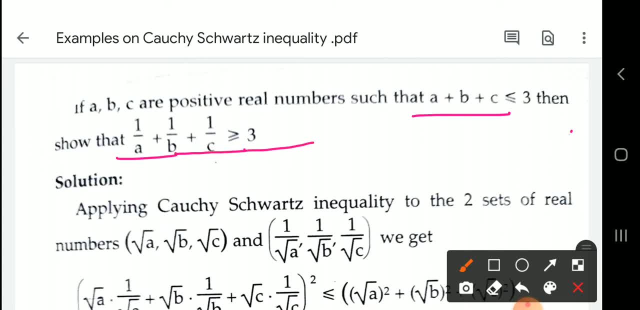 Then we have to show that 1 upon A plus 1 upon B plus 1 upon C, This term is greater than or equal to 3.. Okay, For this example, we again use Cauchy-Squad's inequality. Here we use Cauchy-Squad's inequality for the two sets which are root A into root B, into root C. 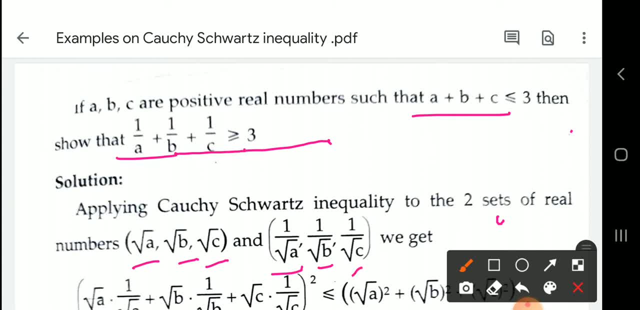 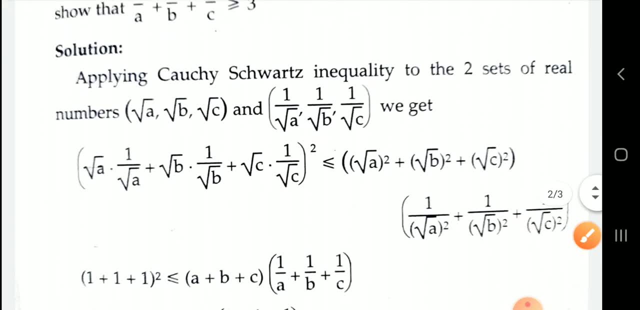 And 1 upon root A, 1 upon root B and 1 upon root C. Okay, For these two sets we use Cauchy-Squad's inequality. So our LHS is summation I running from 1 to N: A, I, B, I, square. 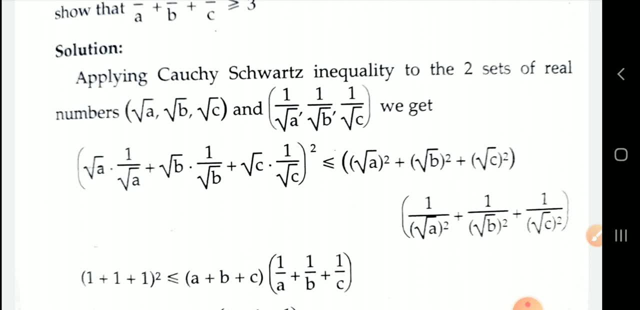 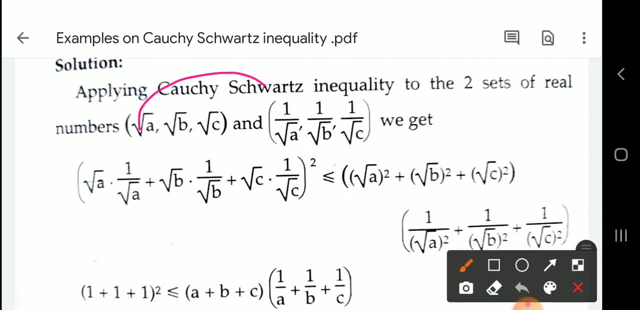 That means A1, B1 plus A2, B2 plus A and B and bracket square. So A1, B1, that means root A, root A into 1 upon root A plus root B into 1 upon root B plus root C into 1 upon root C, bracket square. 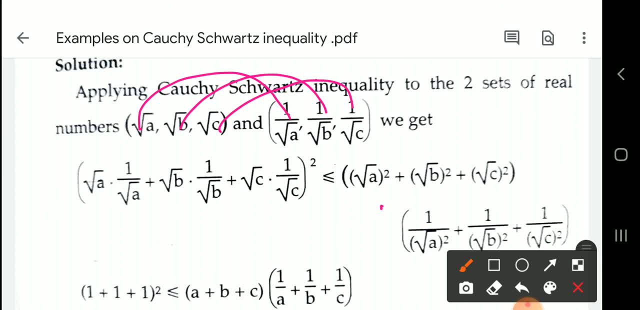 This term is less than or equal to here. First term is summation. I, running from 2 and A, I square That means root A square plus root B square plus root C square into second bracket, sum B. I square 1 upon root A. 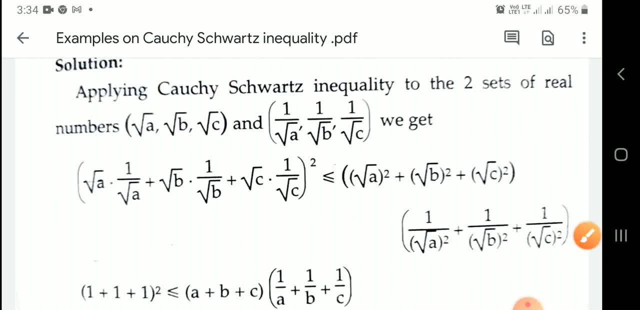 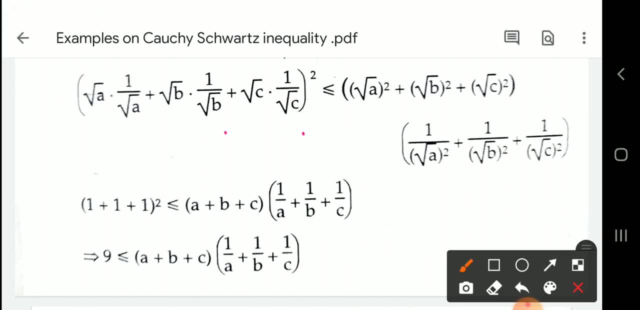 A square, 1 upon root B square and 1 upon root C square. Okay, So after solving this, we get here: root A into root A will cancel. Here, root B into root B is cancel. Root C into root C will cancel, since it is multiplication. 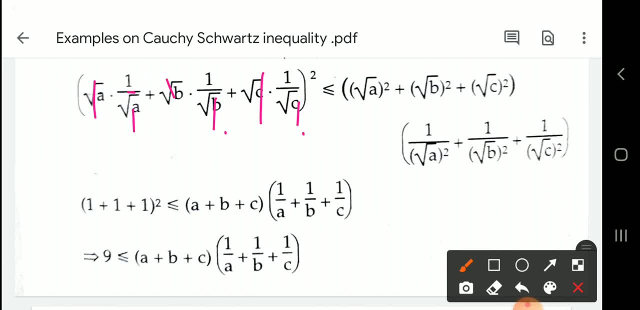 Here 1 plus 1 plus 1, that means 3.. 3 square, 1 plus 1 square. This term is less than or equal to. here Root A square is A, Root B square is A, since square and square root will cancel. 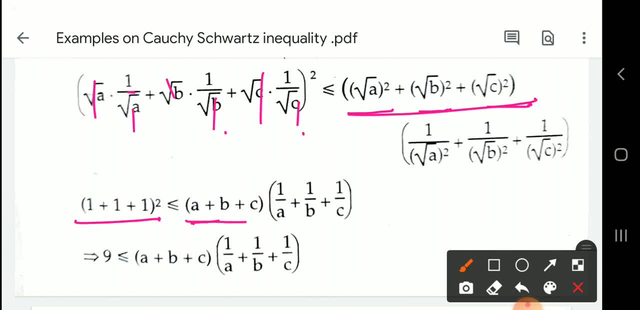 So we get here, after simplification: A plus B plus C, A into 1 upon A, plus 1 upon B into 1 upon C. Okay, So 1 plus 1 plus 1, that is 3.. 3 square is 9.. 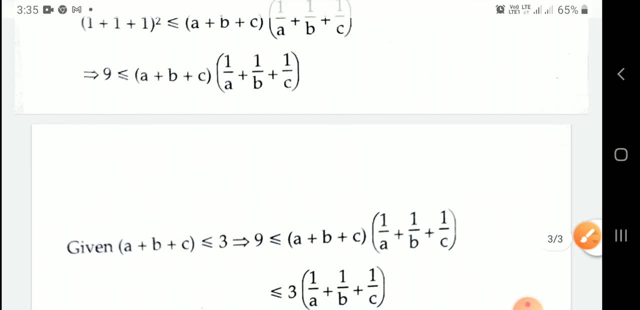 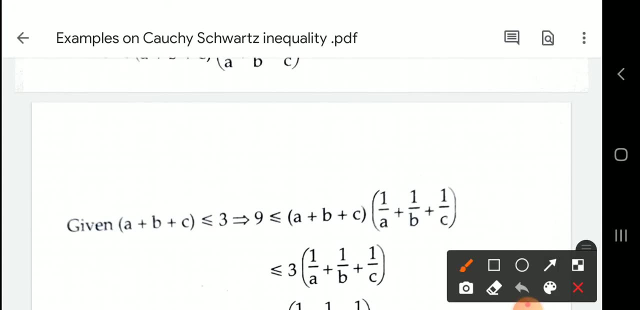 9 is less than or equal to A plus B plus C upon 1 upon A plus 1 upon B plus 1 upon C. Okay, But we have given that A plus B plus C, this term is less than or equal to 3.. 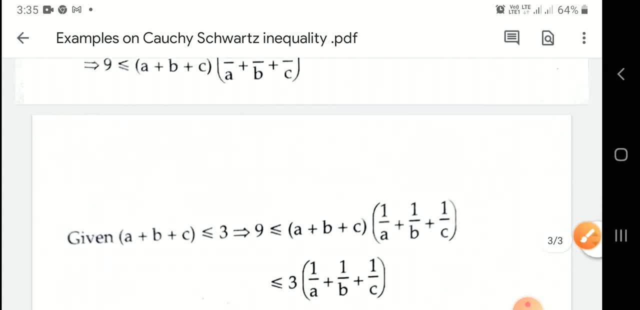 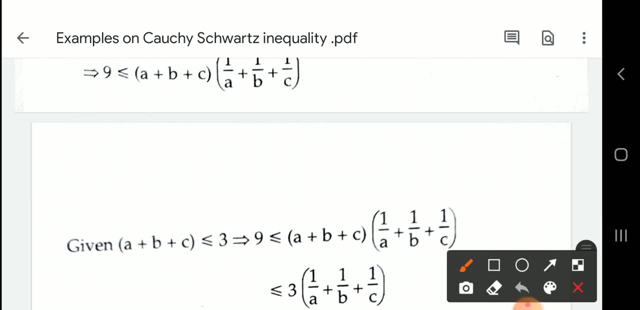 A plus B plus C. this term is less than or equal to 3.. Which Which implies 9.. And we get that 9 is less than or equal to A plus B plus C into 1 upon A plus B plus 1 upon A, plus 1 upon B plus 1 upon C. 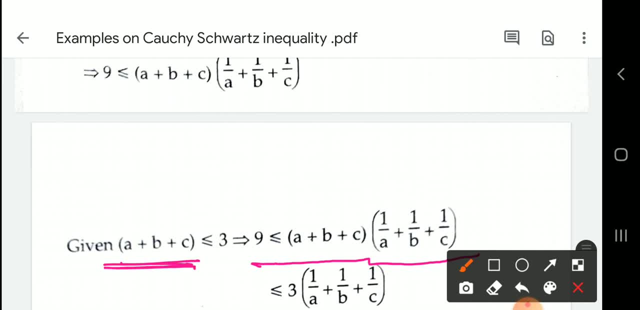 But that term A plus B plus C is less than or equal to 3.. Okay, So for this term A plus B plus C- we use this term- is less than or equal to 3.. For this term A plus B plus C- we use this term- is 3.. 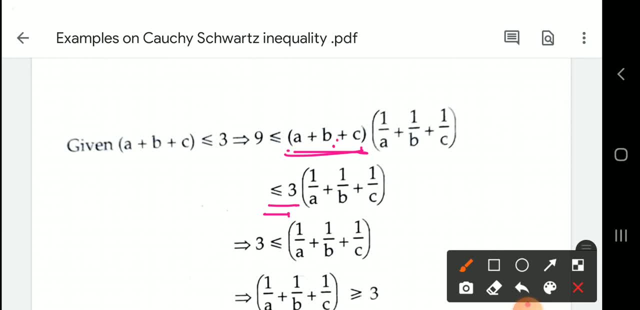 Less than or equal to 3: 1 upon A plus 1 upon B into 1 upon C. This term is same. So we get that 3 is 3 is less than or equal to. here we get, which implies 3 is less than. 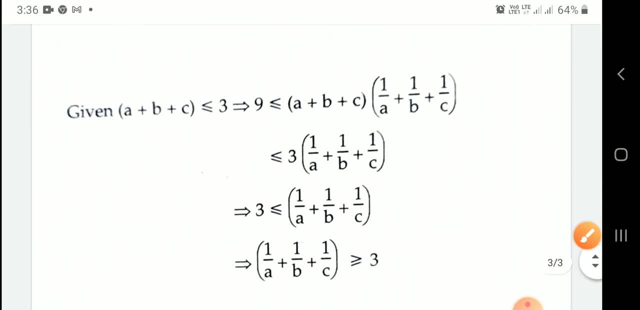 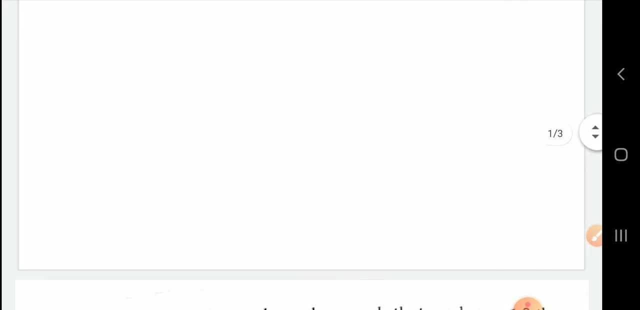 or equal to 1 upon A plus 1 upon B plus 1 upon C, which implies 1 upon A plus 1 upon B plus 1 upon C is greater than or equal to 3.. So we get that 3 is less than or equal to 3.. 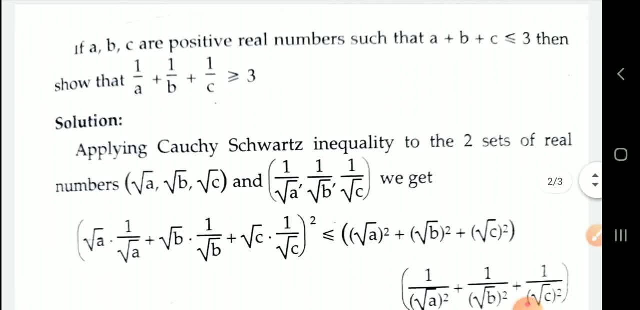 So we get that 3 is less than or equal to 3.. So we get that 3 is less than or equal to 3.. So here we use only the Cauchy-Scott's inequality. So you have to remember the statement of Cauchy-Scott's inequality, which is useful. 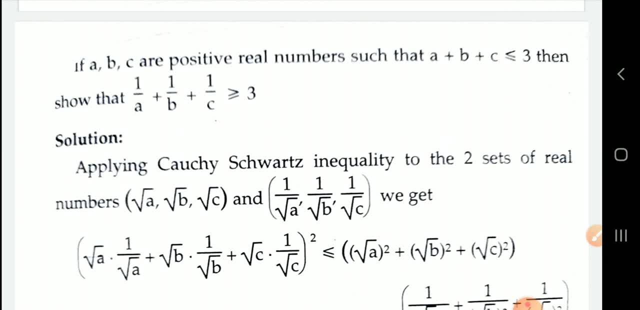 to solve various examples of this type. Okay, Thank you, Thank you. So we're asked to write an expression to represent the perimeter of this figure. So keep in mind that there are four sides. Okay, so you have a measurement of the length for 2x plus 3.. That also means that you have another measurement up top, at 2x plus 3.. Same for the height of x minus 1.. And then you have to understand that there's another measurement parallel to that. 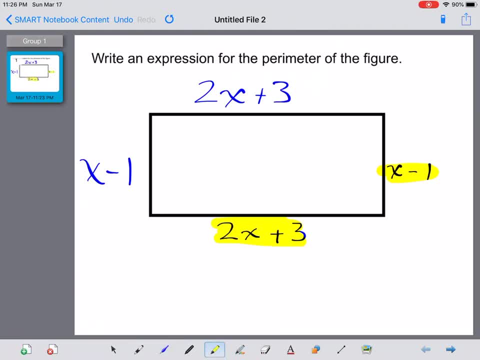 As well x minus 1.. So how do we represent the perimeter? All we have to do is combine all of the like terms, So we have 1x, 2x, 2x and another 1x. That gives us a total of 6x. And for our constants we have a 1 or negative 1, I should say another negative 1.. So that's negative 2..